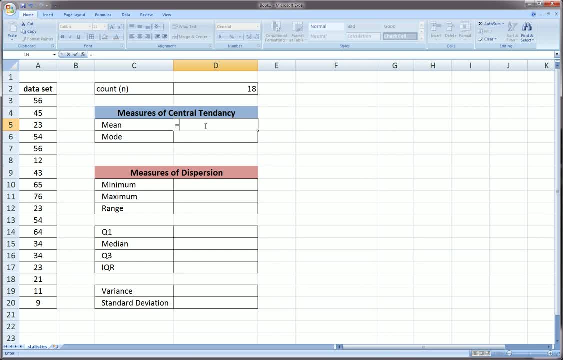 Okay, so let's go ahead and get all these values here. But the important thing is, here all these things are covered, So mean is just average, right. And then we highlight the observations again and it gives us our average Mode is just mode. And of course we put an equal sign before all these functions. 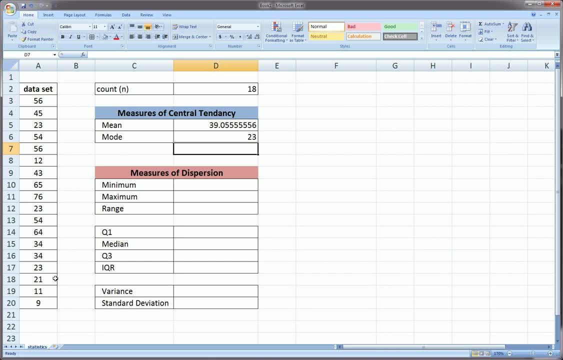 Highlight the observations. and we got our mode And we can see 23 is repeated three times more than any other And that's by definition What the mode is right For. minimum. we got equals min function. Highlight the observations. 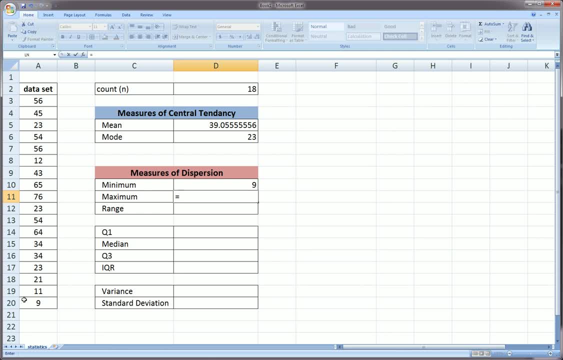 For each one of these functions. we're just highlighting all the observations. For max, it's just max, And to get the range there isn't a function, an easy function. The easiest way is to just take the max, subtract it by the min. 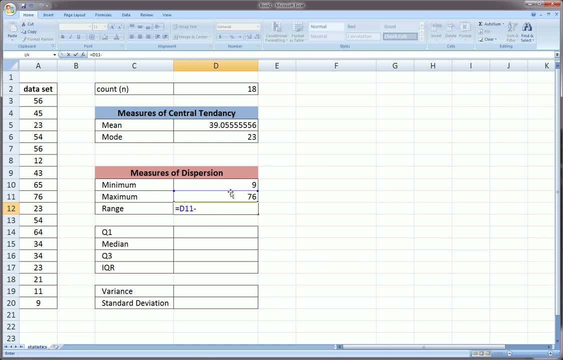 So equals max minus Min right. So 67 is our range Right First quartile. this can be a little difficult to calculate by hand, So luckily Excel has a function for that. It's quartile. You highlight the observations. 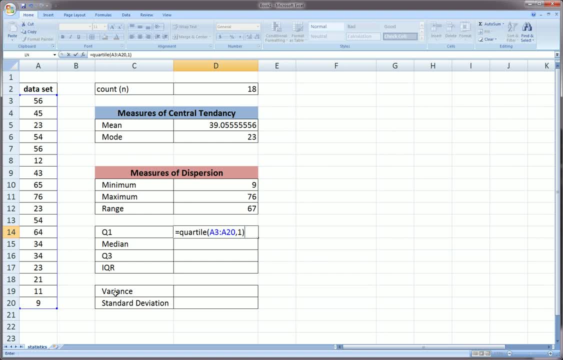 Comma one means I want the first quartile. Okay, so the syntax is: highlight the observations and then comma: what quartile do you want? And for Q1.? Obviously we want the first quartile. The median will be. there's two ways to do this. 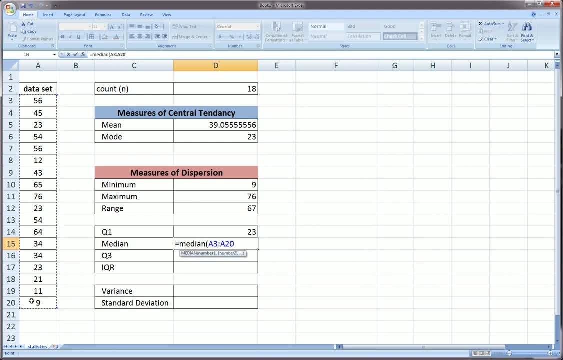 There's a straight median function which you just highlight and enter, Or- and I'll do this on the side so you can see we get the same result. You could use quartile again And this will illustrate the point I made earlier. 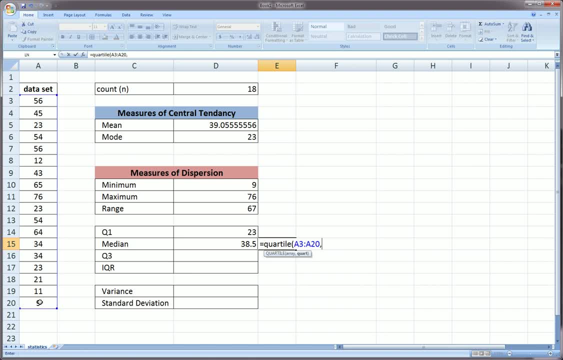 You highlight all the observations, Comma this time. Median, we know, is the second quartile And you see, We get the same result. okay, Now for the third quartile. you guessed it, We highlight it. 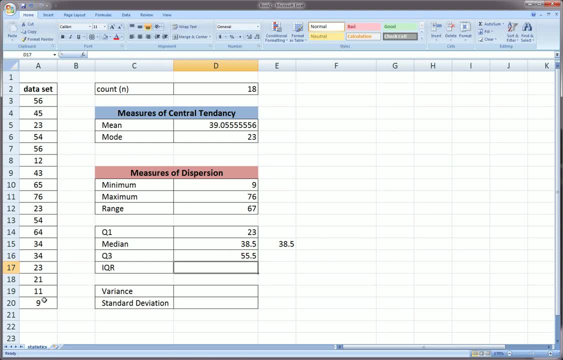 And then it is three Comma, three right, And for the interquartile range which some of you will be asked to calculate, it's just the third quartile subtracted by the first quartile, And what that basically means is that 50 percent of the observations are. 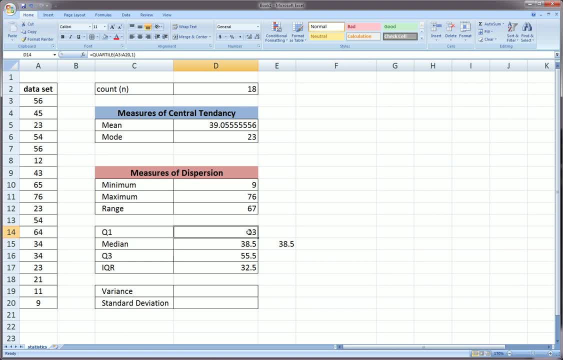 between 55.5 and 23,. right, And the range of that is given by this IQR interquartile range And for some really common measures of dispersion, variance and standard deviation which are very cumbersome to calculate by hand. 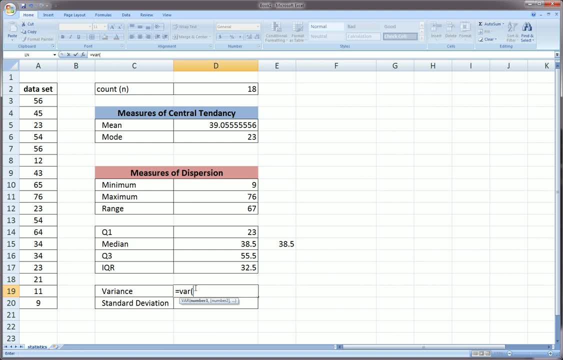 here there's a function called just var, And make sure you don't use var p, because that's for population variance. Here we have a sample. It's very important because in the sample variance formula we divide by n minus 1. And in the population variance we divide by just n. 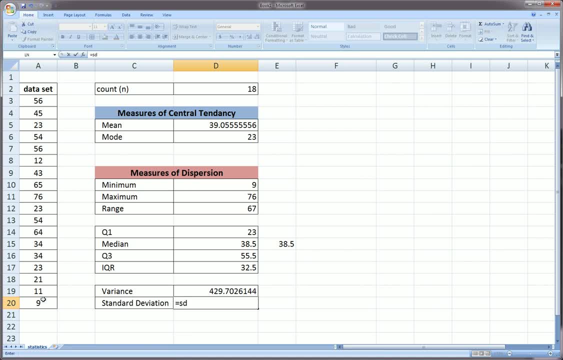 And the same thing goes for standard deviation. Make sure you use SD and not SDP for the same reasons cited. Actually, sorry, it's STD, STD, STD, STD, STD, STDEV, STDEV, STDEV And not STDEVP, right? 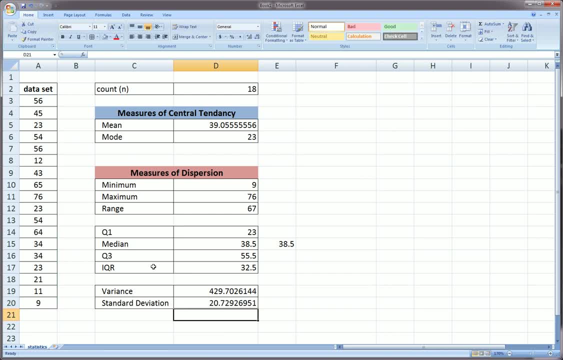 Because this is a sample. Okay, And just to brush this up and make it all look good, we can highlight this entire column and get rid of some of these extra decimal places by using the reduce decimal place button over here. Make them two. 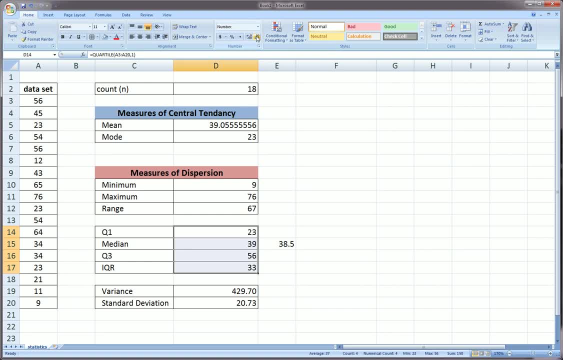 And you can highlight, You can increase, You can decrease Decimal places As you wish, Just to make everything look clean. Okay, So here's some basic descriptive statistics on a basic data set, on a basic sample, And I hope you learned something from this. 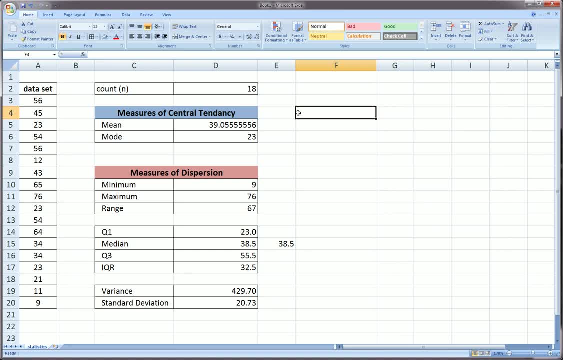 A bunch of functions Really straightforward but really useful. And make sure you check out my channel, RD Gelayer, And subscribe, And I'll see you next time. Bye, Bye, Bye, Bye, Bye, Bye, Bye.